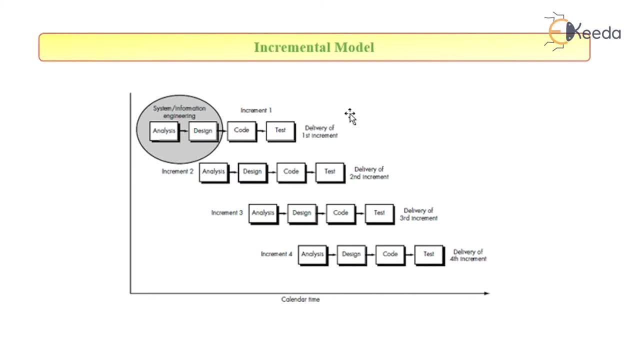 products in increments. That means, unlike the waterfall model, where all the requirements are gathered right at the beginning and then the designing of the entire software takes place at one go- sure, one increment or one part of the module or of the software is being worked out. After that it is being delivered to the user If they seek an approval. 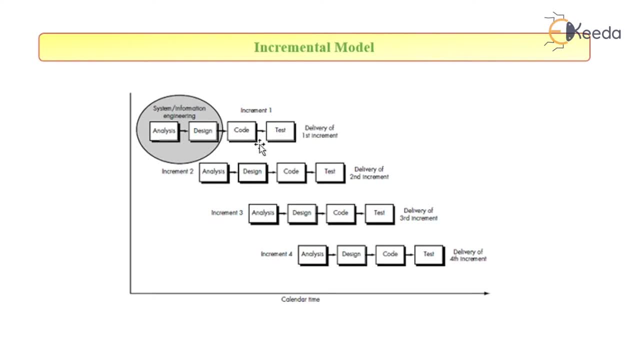 from the user. it has been incremented or it has been developed, with the next stage of the process and then the delivery of the second increment takes place. For example, if there is a social media site which is to be created once the login page is created, then it has been. 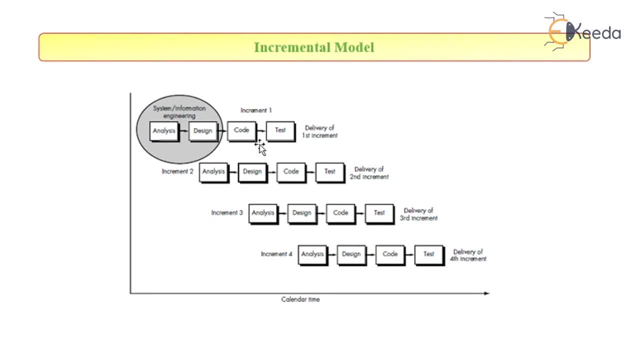 delivered to the user. That is the first increment. Once approval is seeked from the user, the login page is incorporated with the about myself page, which will be my second increment Now. these two increments are then incremented, or then combined with the friends page so that the three increments 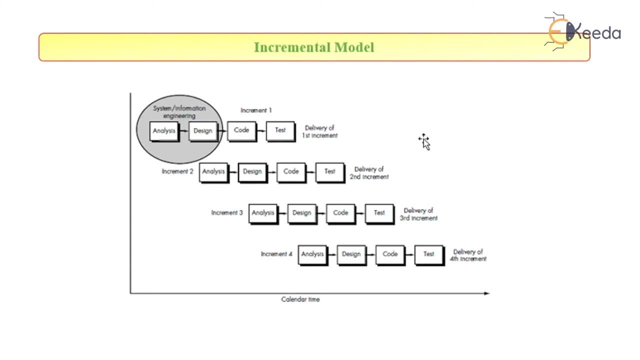 are ready for the next level in order to complete the project in the form of increments. One increment is delivered- seek approval, then deliver, make. and deliver the second increment- seek approval, make the third one, seek approval, then it is a final delivery of the entire software. 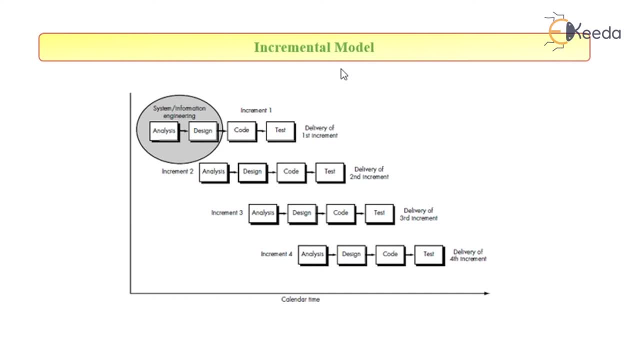 The phases included are analysis, design, coding and testing. Analysis phase consists of gathering of requirement. This phase is the one initiation phase in which there is a basic communication about the product or project between the customer and the user. The needs of the project are: 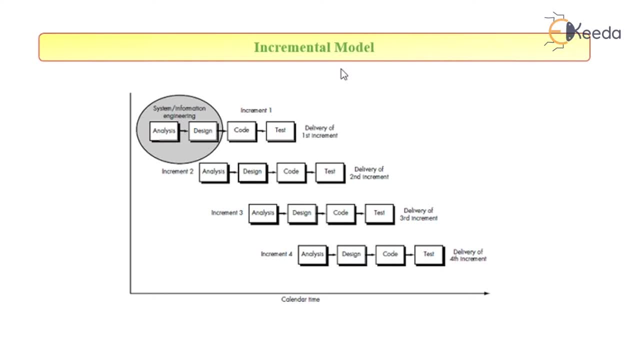 identified, the problem statement is defined, the scope of the project is discussed between the customer and the user. After that, planning is taken place. Planning involves cost estimation, budget estimation, scheduling of the resources, and then we move on to the next phase, which is the design phase.